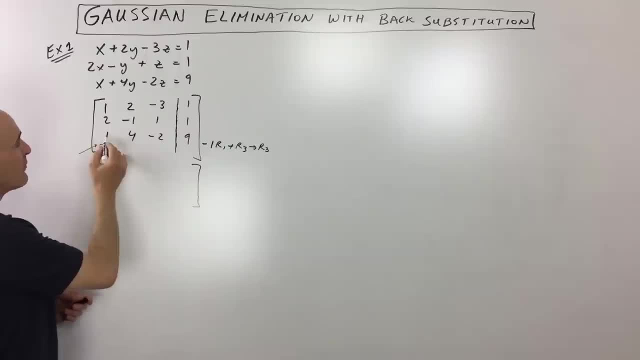 but let me see if I can show you. So negative one, okay plus one gives us zero. negative two plus four is two. positive three plus negative two is one and negative one plus nine is eight. Okay, the other two rows are staying the same, so I'm just going to copy those down as they were, okay, and let's see. 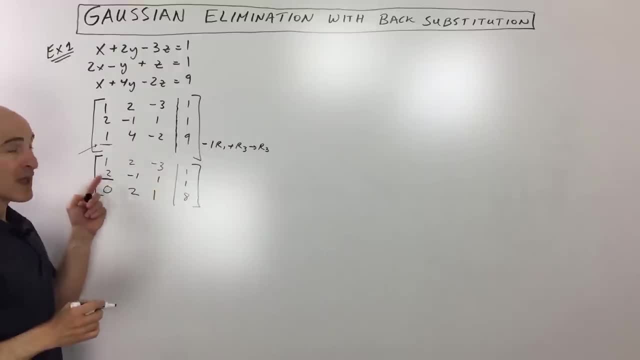 So now the next step is: we want to get zero in this position right here, and the way I'm going to do that is I'm going to multiply negative two times row one, I'm going to add that to row two and I'm going to put the answer in row two. 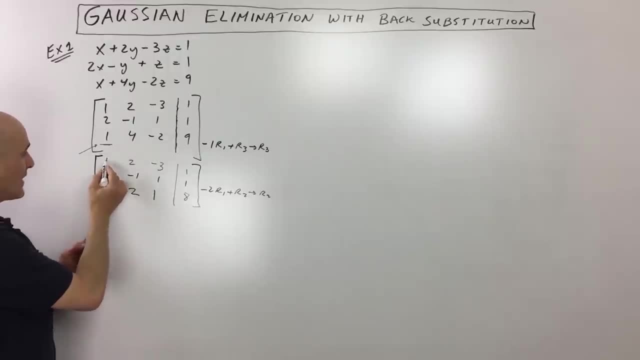 Okay, so let's go ahead and do that. Now we're going to multiply negative two times one, which is negative. two plus two is zero. Negative four plus negative one is negative five. Six plus one is seven and negative two plus one is negative one. So you really have to be careful with that. 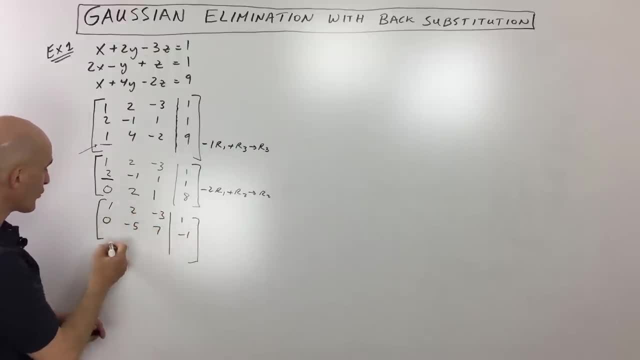 arithmetic, because if you make a little mistake, it's going to throw the whole system off. Okay, so now we've got zero in these two spots Here. our next step is to get zero right here. Okay, and the way that I'm going to do that is: 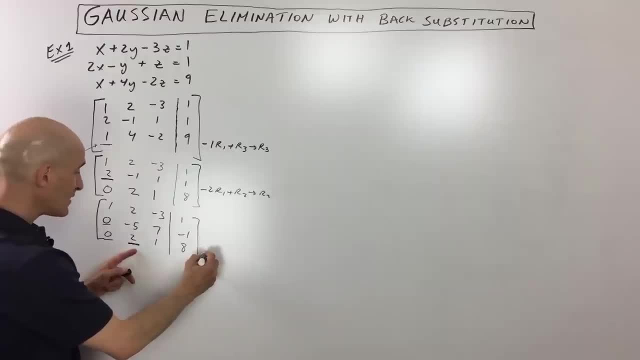 I'm going to multiply the row two by two, So two times row two, and then I'm going to add it to five times row three. I'm going to put the answer in row three. Okay, so you're with me. so far, So. 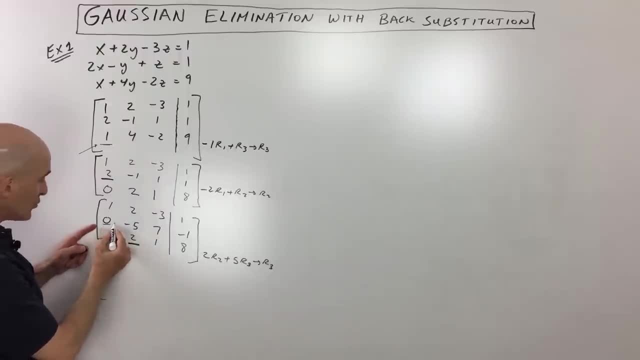 let's go ahead and do that. So we're going to say two times row two: Okay, so that's going to be zero. and then this is going to be, let's see, negative ten Plus positive ten. that's going to give us a zero. Okay, good. And then this is going to give us. 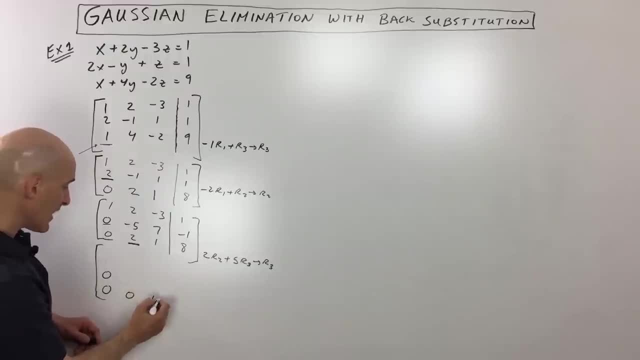 fourteen plus five is nineteen, right. And then over here we've got negative two plus forty, which is thirty-eight. Okay, now the other rows, they don't change, They're staying the same. So I'm just going to copy those down. It's a lot of a lot of writing, but the nice thing is you don't. 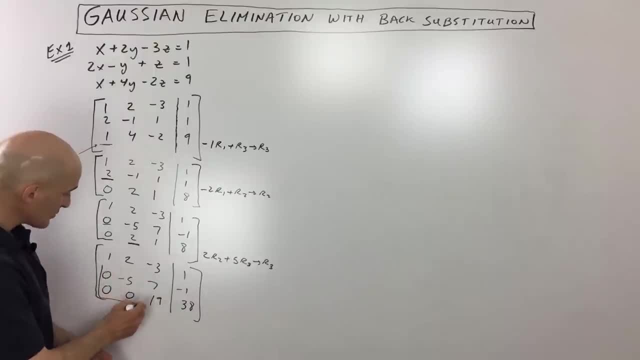 have to write the variables over and over again. So now you can see we've gotten zeros here in this lower left hand corner. So now we're going to copy those down. So now we're going to copy those down. The next step is: you want to get ones on the diagonal. Okay, so with me so far. you want to get? 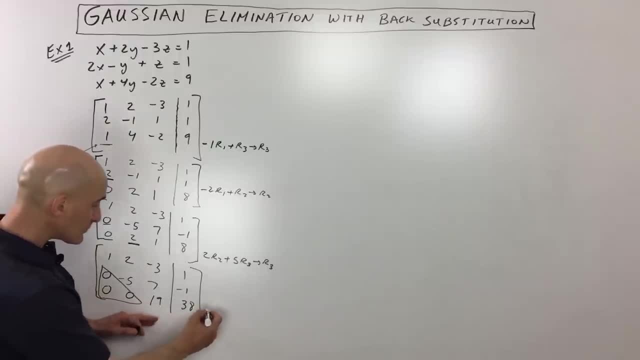 ones on this diagonal. So what I'm going to do is I'm going to multiply one-nineteenth times row three. I'm going to put that answer in row three. I'm also going to multiply negative one-fifth times row two and I'm going to put the answer in row two. And then the first one is already starts. 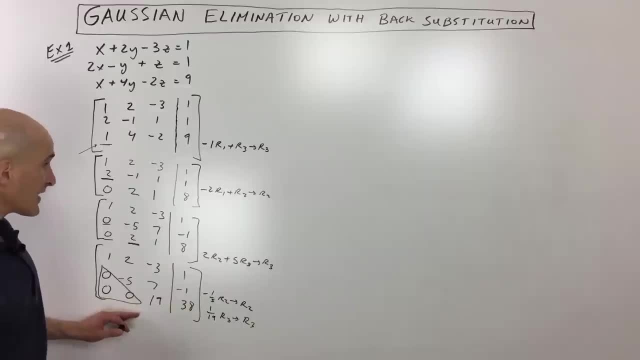 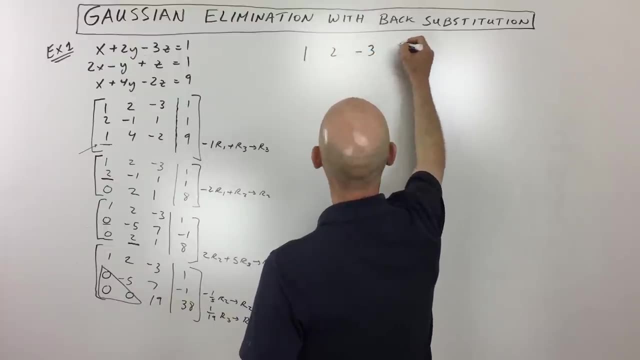 with a one. so we're good there. So let me go ahead and do that next step here. So that's going to give us. Let's see, what do we have here? We've got one, two negative-three, one okay, and we've also got zero one and let's see negative seven-fifths and 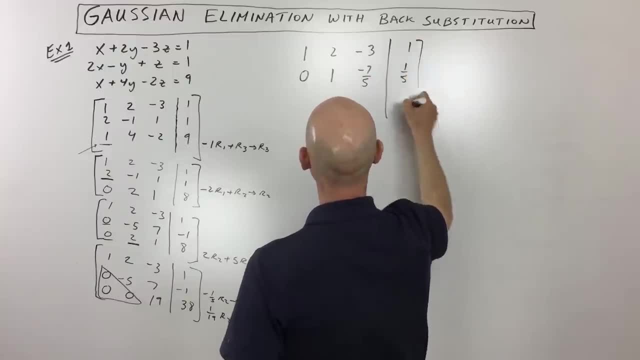 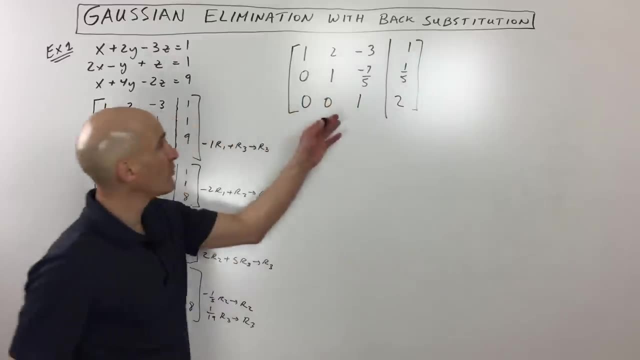 we're multiplying by negative one-fifth. this is one-fifth, and let's see what else we have. we've got zero, zero, one and two. okay, so now, if you can see what we've got so far, this, we are going to rewrite these. 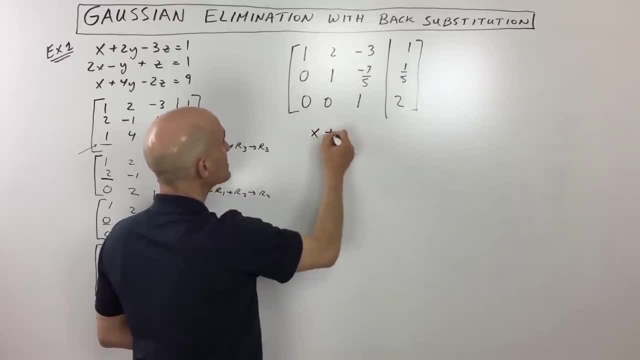 as equations now. so this is actually the top equation is 1x plus 2x, two y minus three, z equals one. The second equation is zero x plus one, y minus seven, five, z, seven, fifth, z equals one, fifth. And the last one is one z is equal to two. 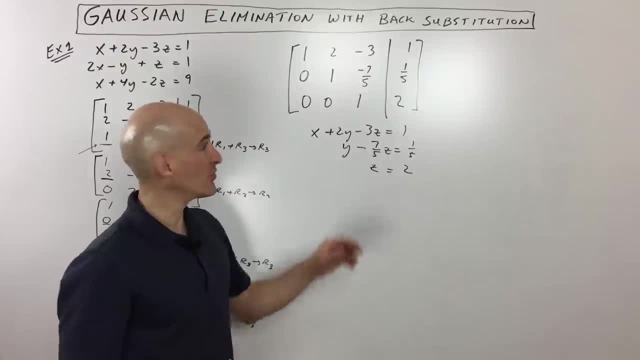 So now here's where the back substitution comes in. You see this kind of stair-step pattern. We've got one variable, one equation. You know, we've got the second equation. we've got two variables. The top equation's got three variables. 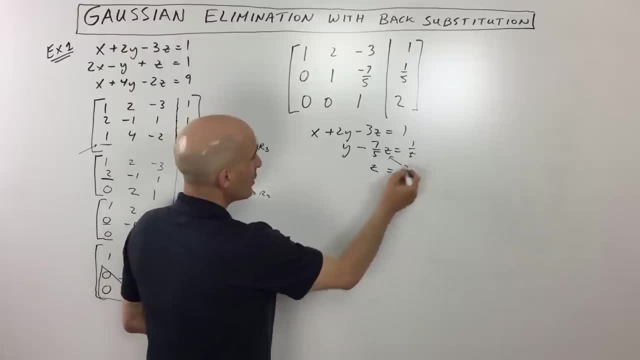 So we're just gonna back substitute. So if I put two in for z, okay, we already know what z is. We've got y minus seven fifths times two equals one fifth. So that's gonna be y minus 14 fifths equals one fifth. 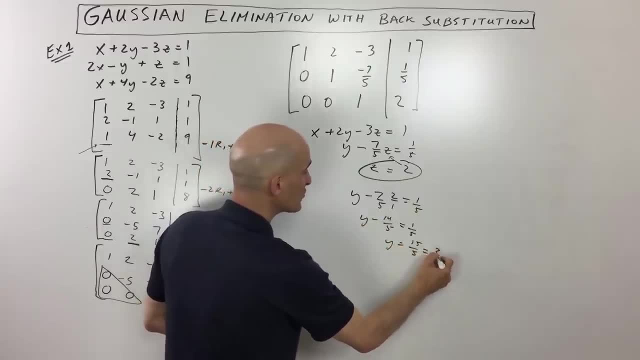 And if we add the 14 fifths to the other side, we get 15 fifths, which equals three. Okay, so now we know what z and y are. We just have to solve for x. Let's go to the top equation. 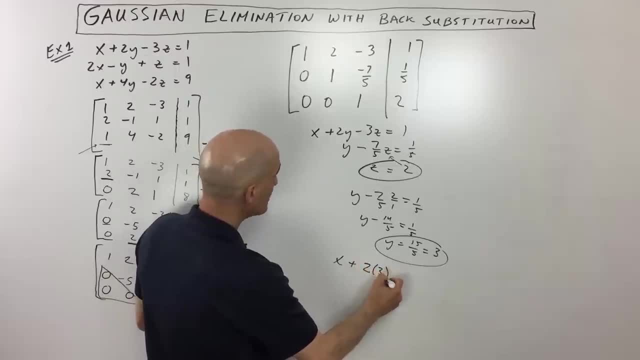 We've got x plus two times three, because that's what y is minus three times two, That's what z is equals one. So we've got x plus six minus six is equal to one. The six and the negative six cancel. 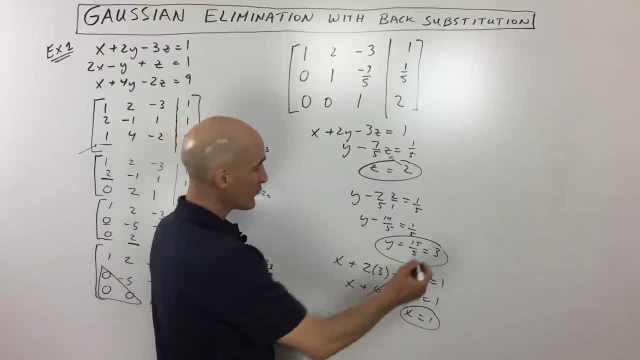 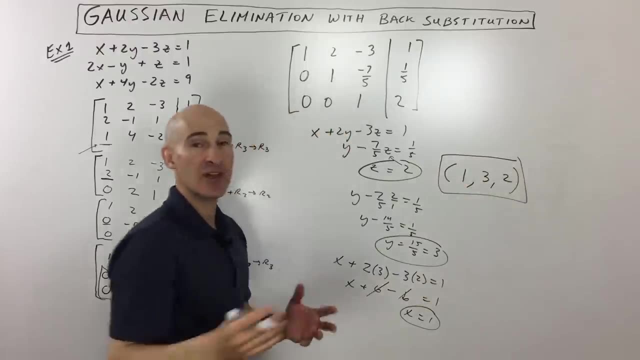 so you can see: x equals one And if you wanna write your final answer, you would write it as a triple: X is one, y is three, z is two. That's your answer, And then you can check your answer if you want. 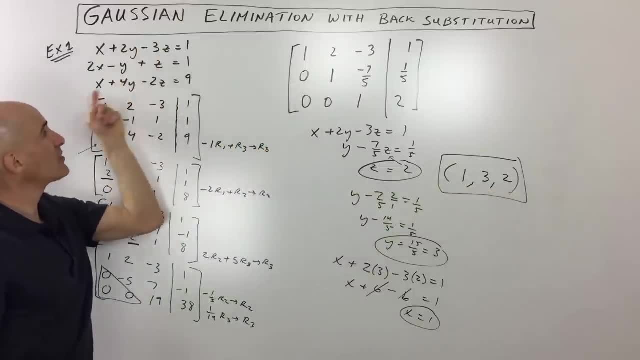 by taking these values x, y and z, putting them into all three of the equations here, making sure that they give us the appropriate solutions on the right. So again, this is Gaussian elimination with back substitution. We're gonna go through another example. 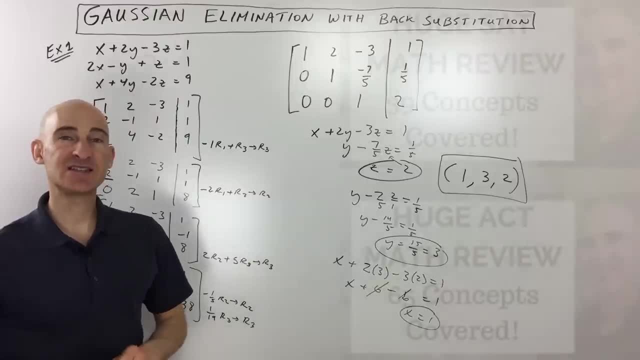 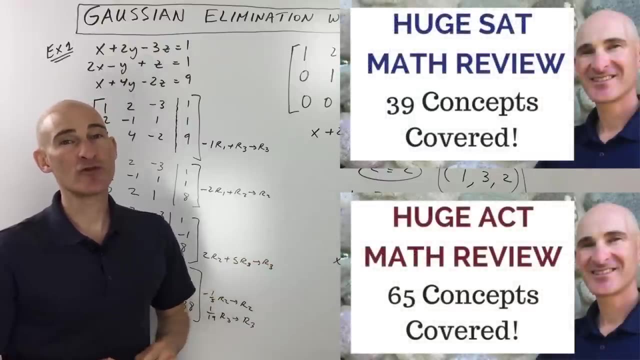 to show you more how it works. But before I do that, if you're preparing for the ACT or the SAT, check out my huge SAT math review video course and my huge ACT math review video course. They go through a lot of different concepts. 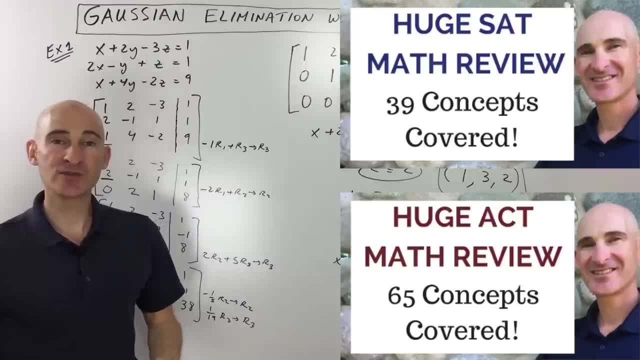 We have a teaching segment. There's opportunities to practice and do some problems, And it just gives you a good overall review and an insight into some of the key things that they want you to know when you're taking that test. So definitely check that out. 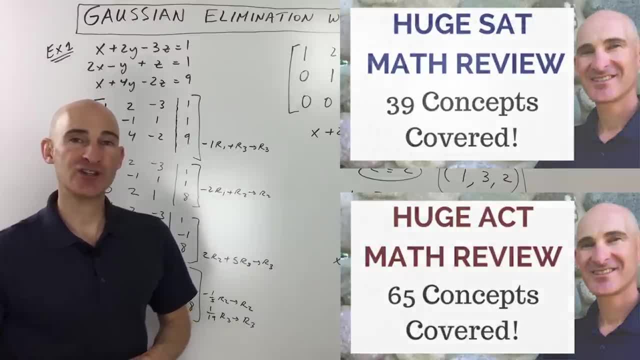 I have a link below in the description, And also you can check out the links through my About page on my YouTube channel, Myers Math Tutoring. But let's get into the next example. Let me erase this board and I'll be right back at you. 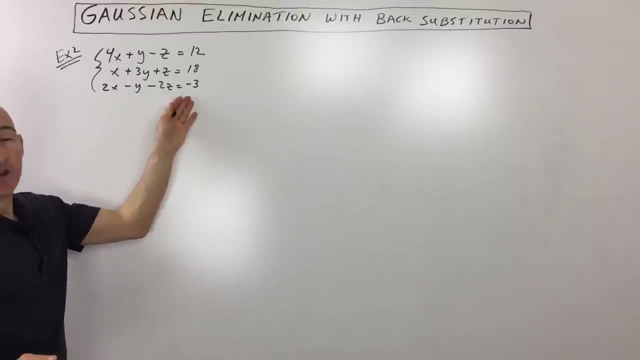 Okay, example number two. You can see we've got a three by three. okay, three variables, three equations, And the first thing we wanna do is we're at our augmented matrix. So let's go ahead and do that. So we're just using the coefficients. 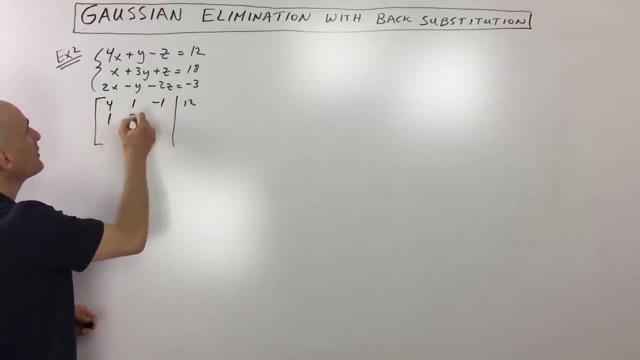 the numbers in front of the variables, right, And let's see one, three, one, 18.. We've got some larger numbers here, so we might have to take out the calculator to do some of these calculations. okay, to make it go a little bit quicker. 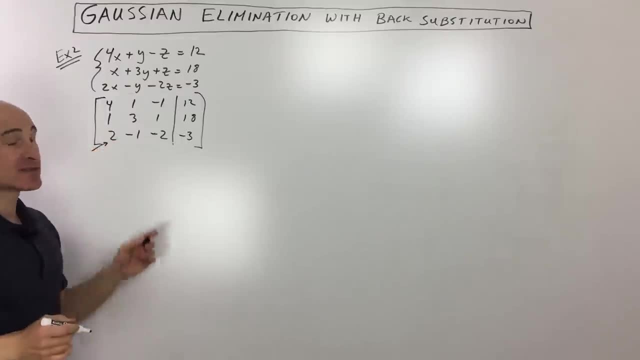 But remember, our first step here is to get zero in this lower left-hand corner, And the way we do that is we wanna combine either the first with the third or the second with the third. I'm just gonna take negative two times row two. 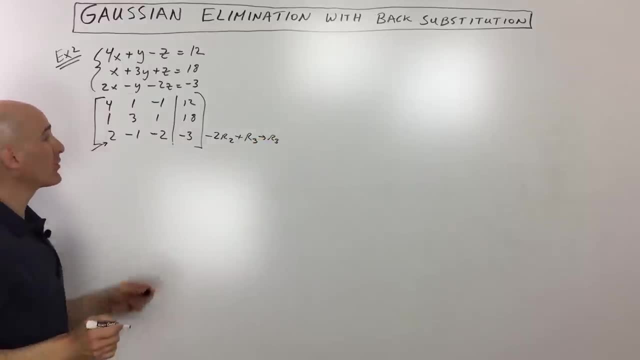 plus row three, and I'm gonna put the answer in row three. Okay, so if we do that, I'm just gonna copy down. I usually like to kinda write down the rows that haven't changed, just to kinda get that out of the way. 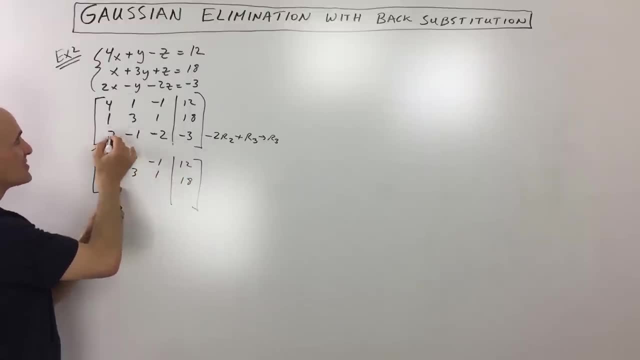 And so now this is the row that's gonna be changing, row three. So negative two times one is negative two plus two is zero. Negative six plus negative one is negative seven. Negative two plus negative two is negative four And negative 36 plus negative three is negative 39.. 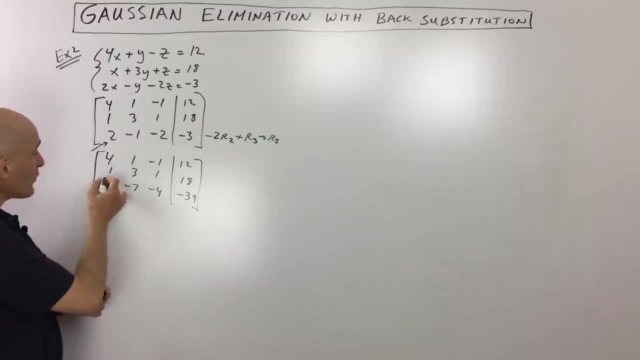 Okay, so you can see the numbers are getting large here. Okay, the next step: we wanna get zero right here where that one is, And so what I'm gonna do is I'm gonna combine the first equation with the second equation, So that's gonna be negative. 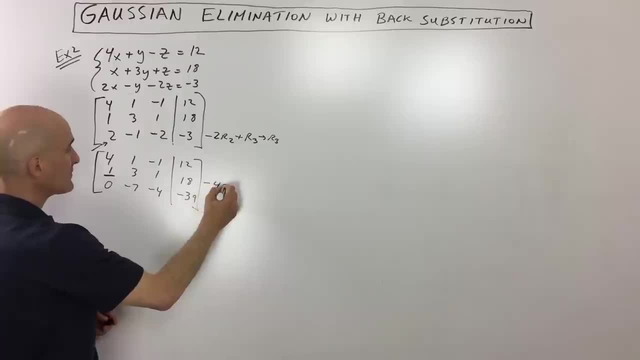 let's see negative four times, row two plus row one. answer goes in row two. All right, so let's go ahead and do that. So we've got. let's see a copy down this bottom row, because that's not changing. 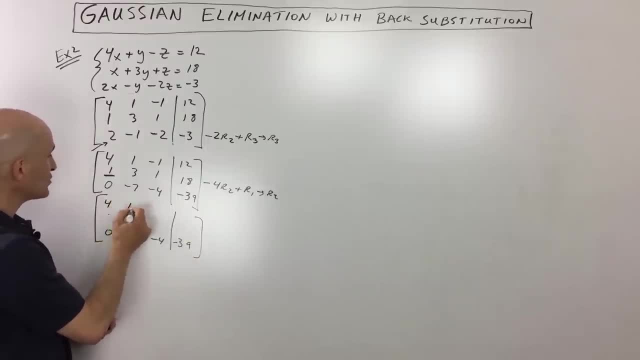 Yeah, and again, be careful that you don't make little simple mistakes, because that's easy to do with this method. Okay and so let's see. So we've got negative four times this row plus this row. So that's gonna give us zero. 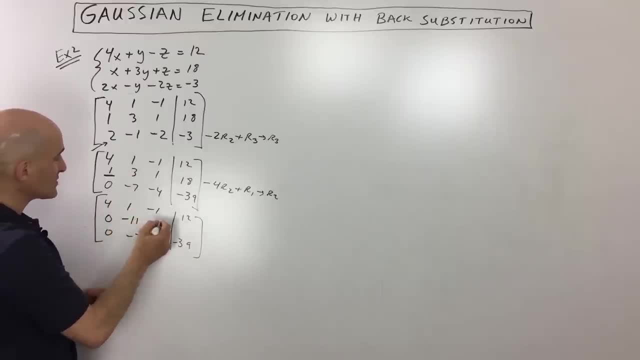 Negative 12 plus one is negative 11.. Negative four plus negative one is negative five. Negative four is gonna give us negative 72, plus the 12 is negative 60.. Okay, so now we've got zero in this spot, This spot. now we wanna get zero over here. 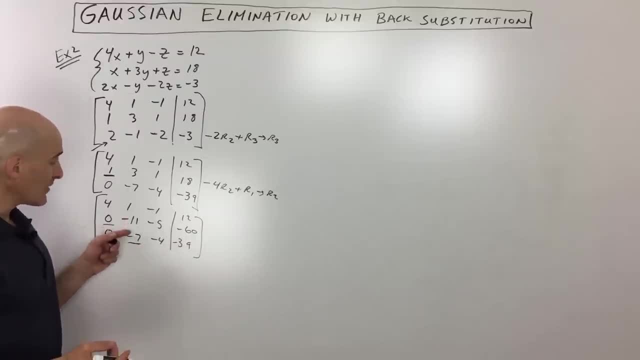 where the negative seven is. And so the way I'm gonna do that is I'm gonna combine the second row with the third row. Now you might be thinking: well, why aren't you combining the first with the third? Well, if I combine the first with the third, 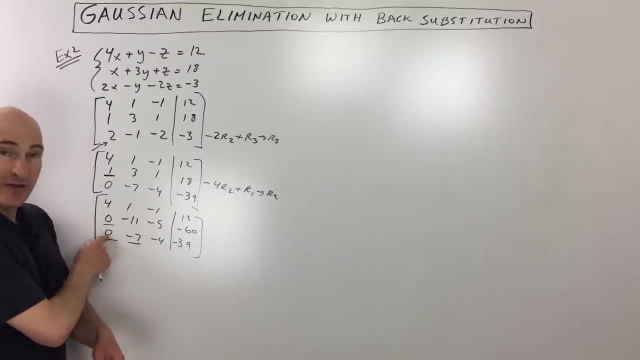 what's gonna happen is you're gonna end up getting a constant besides zero in this lower left-hand corner, which is gonna kind of reverse out what we did earlier when we tried to get zero here. So that's why I'm just combining the second and the third. 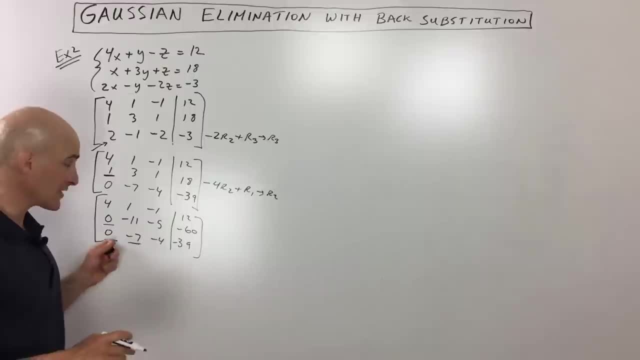 because you can see, when you add zero and zero, that's just gonna still be zero, so it's not gonna get rid of this zero in this place here. So let's go ahead and figure this one out. We're gonna have to. let's see. 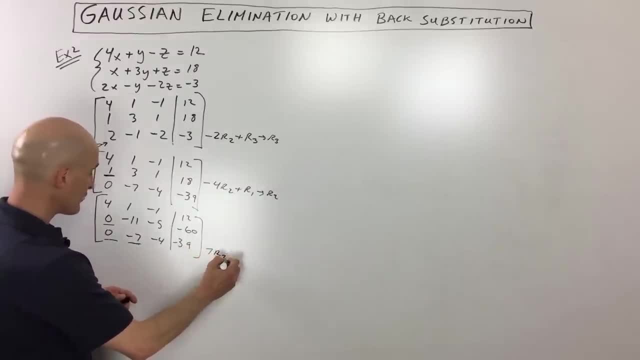 multiply seven times row two, right, plus a negative 11 times row three, and we're gonna put the answer in row three. Okay, so let's go ahead and do that. So we've got four. we've got one. we've got negative one, we've got 12, right? 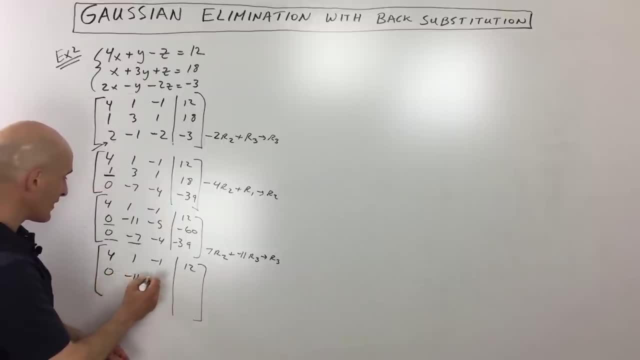 And let's see, this one is gonna stay the same. so zero negative 11, negative five, negative 60.. This one is gonna be, let's see, seven times row two, that's negative 77,, plus positive 77,, that's zero. 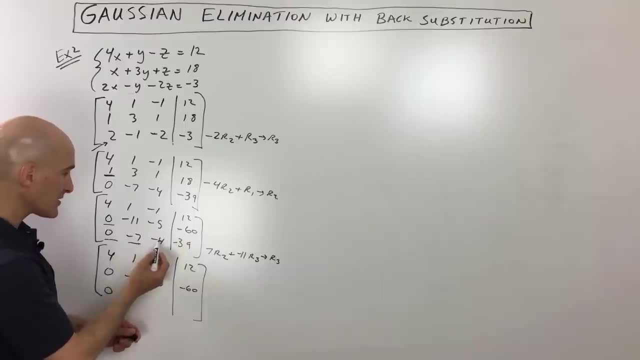 We've got negative 35,, okay, plus 44, which is how much? That's nine, right. And then we've got- let's see, here's where I'm gonna break out the calculator- We've got seven times row two. 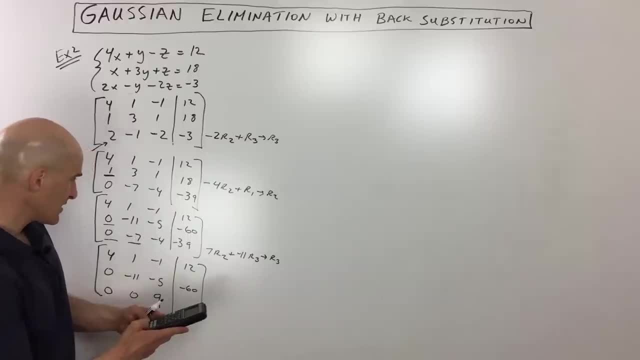 so that's gonna be negative 420,, right, Plus a negative 11 times a negative 39,, which gives us nine. Okay, so that worked out. nice, okay, so there we go. So now you can see we've gotten zeros. 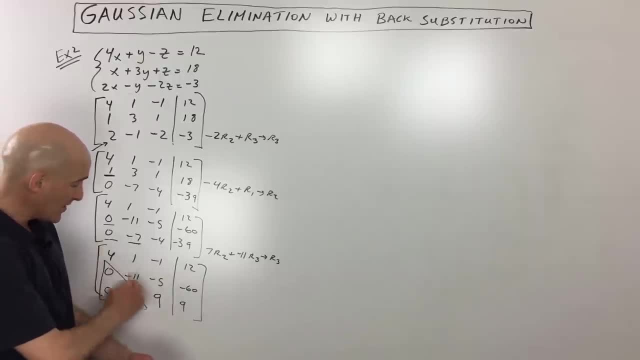 in that lower left-hand corner. The next step is to get ones on the diagonal. okay, So the way I'm gonna do that, I'm just gonna multiply 1 9th times. row three: I'm gonna put the answer in row three. 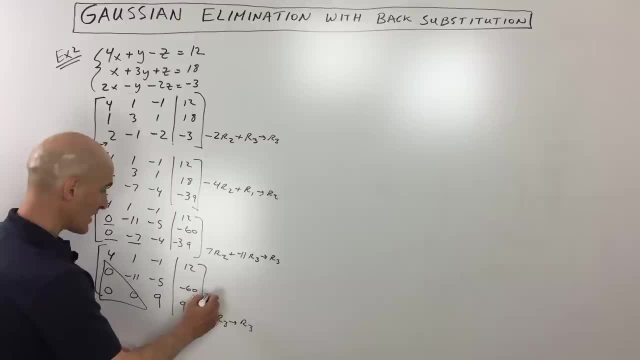 I'm gonna multiply row two times negative- 1- 11th, and I'm gonna put the answer in, of course, row two and then row one. we're gonna multiply by 1- 4th, and I'm gonna put the answer in row one. 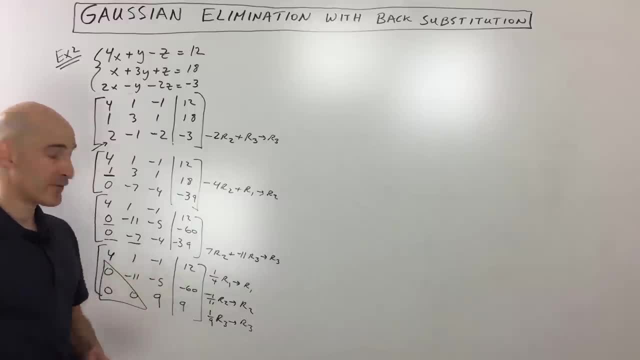 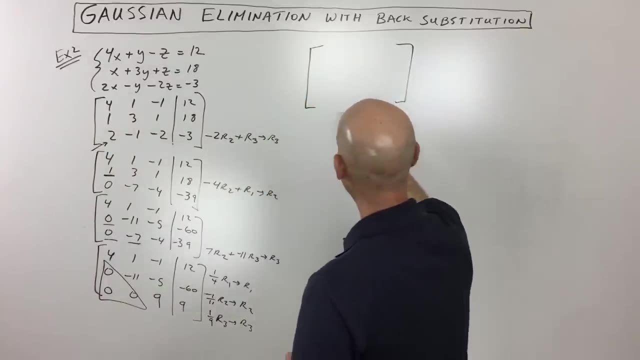 So I'm just multiplying through by the reciprocal of the leading coefficient for that row. So if I do that, let me switch over here now. okay, We've got on the bottom row. we've got zero, zero, one and one. okay. 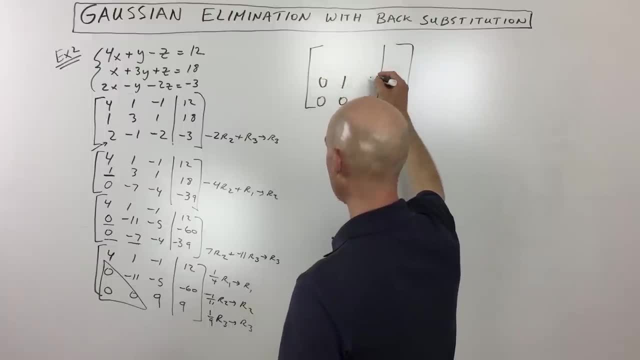 And in the second row we've got zero one. let's see 5 11ths and let's see this is gonna give us 60 over 11, and then we've got one 1, 4th. 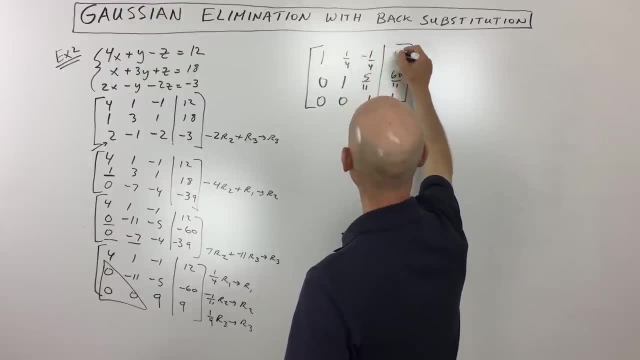 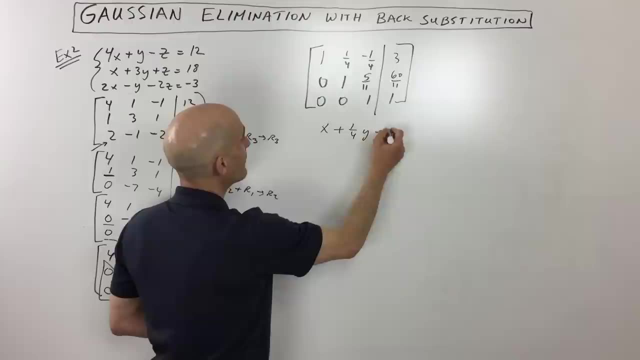 let's see negative 1, 4th and three. Okay, so our equations now are gonna be: let's see, we've got the top row, which is x plus 1 4th, y minus 1 4th. z is equal to three. 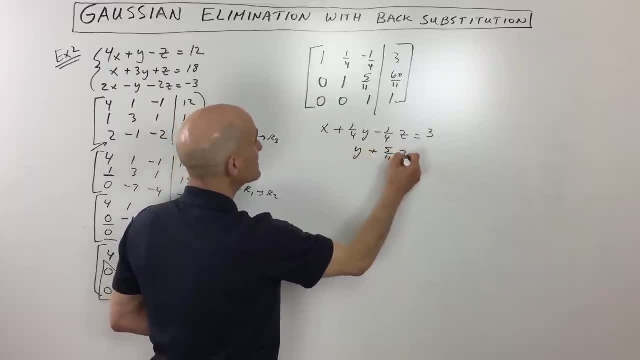 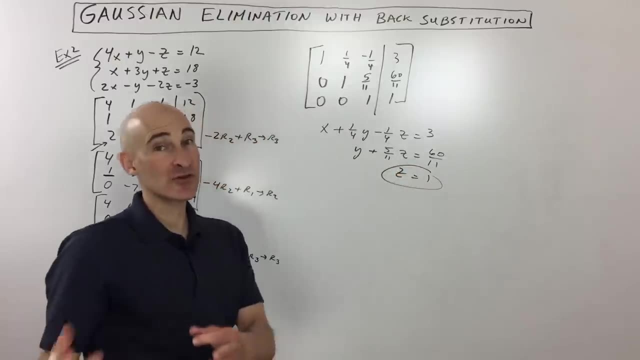 We've got one y plus 5 11ths. z is equal to 60 11ths right. And then the last one. we can see that we have z equals one. So we've already got z solved for, so that's good. 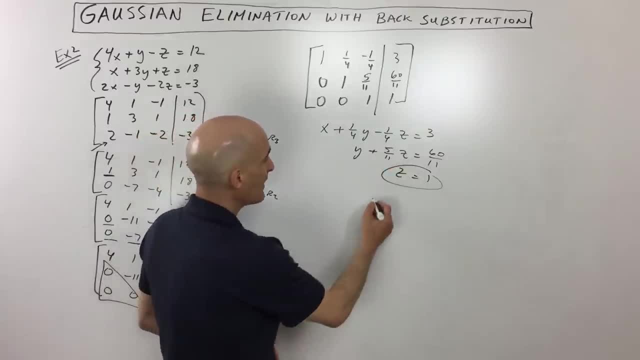 Now we're gonna do our back substitution. So if I put one in for z, that gives us y plus 5 11ths is equal to 60 11ths. Subtract the 5 11ths and that gives us y is equal to 55 11ths, which is equal to five.